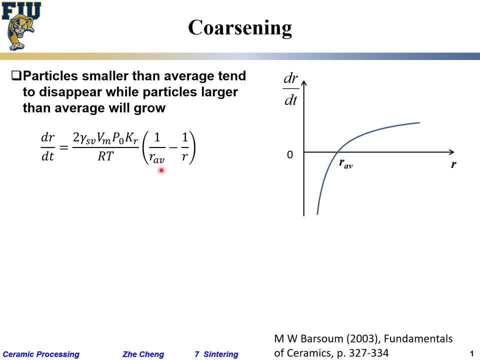 make sense. so what essentially it tells us is: if your radius is average radius, this term become- if your radius is average radius, this whole term become zero, which means you do not change in size. the particle size does not change with time. on the other hand, if you are larger or smaller, it will change, and the kr is a so-called coarsening rate constant. let's 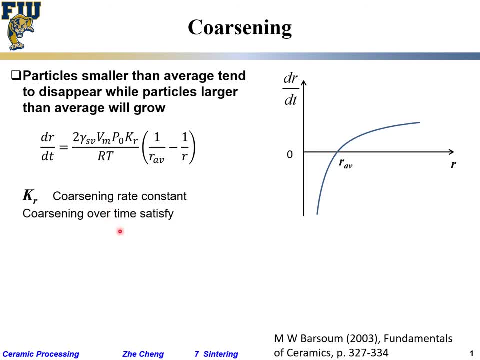 don't go into the detail and the coarsening over time would satisfy what people generally said. observed something like this, a parabolic kind of like a parabolic relationship. the average squared versus initial average is follows this relationship. but anyway, based on this, if my r initially radius is larger than 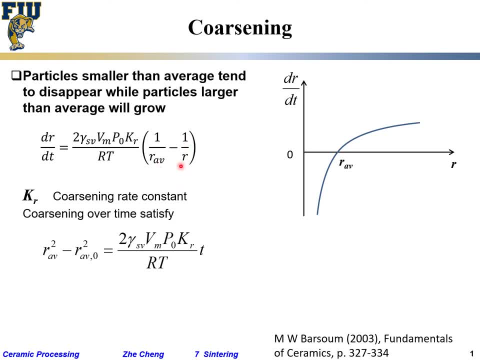 average, which means one over r would be smaller than one over r a v, and then this term: would be well, if r is larger than r a v, this term would be positive, which means the particle would go. that's what we draw right. on the other hand, if r a v is smaller, r a v r is smaller than r a v. 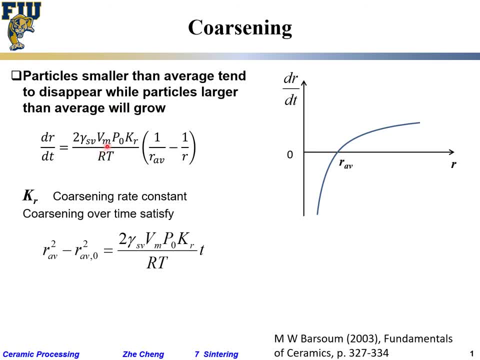 i would have this whole thing be negative. the particles would get smaller and smaller, eventually disappear. that's what we said here. okay, but overall, over time it the whole thing may also change a little bit. follows kind of like a parabolic relationship. okay, coarsening kinetics based on this kinetics, which means how fast does the radius increase? 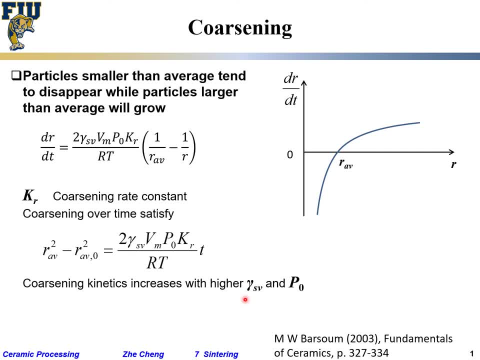 would increase with higher surface tension and as well as higher equilibrium pressure. what does that mean? if your particles has larger surface energy, it has a greater tendency to shrink its surface energy. as a result, the particles tend to cause quickly to reduce the surface energy. at the same time, if p zero means the high variable pressure, high variable pressure is: 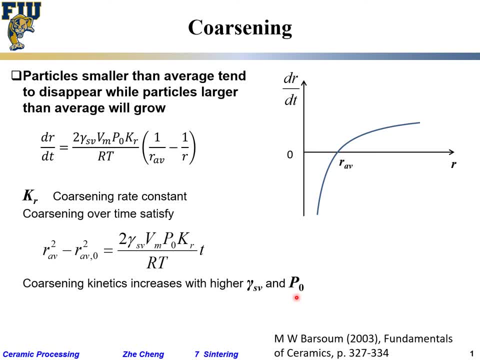 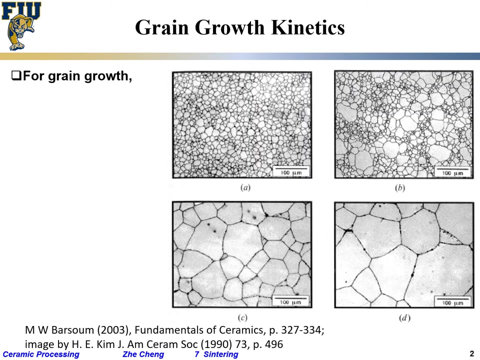 the higher the pressure means it has a greater tendency to go through the vapor phase. the transport is faster, make sense. higher vapor pressure means the transport through the gas phase would be faster and in that case you also have higher green growth or coarsening rate. make sense, okay? so let's look at some micrograph image. i'm not 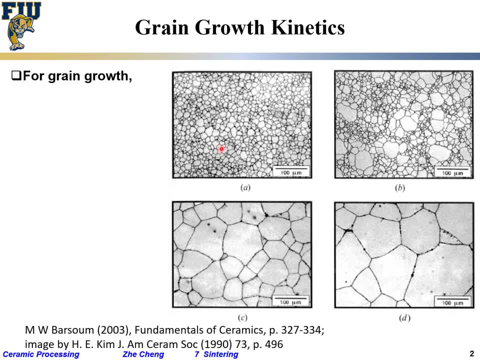 sure what material this is, i have to dig into it. but i'm not sure what material this is, i have to dig out. but essentially you see, initially fine grain. over time some grains get larger, some green appear to be- you look at here- getting smaller and then eventually everything. 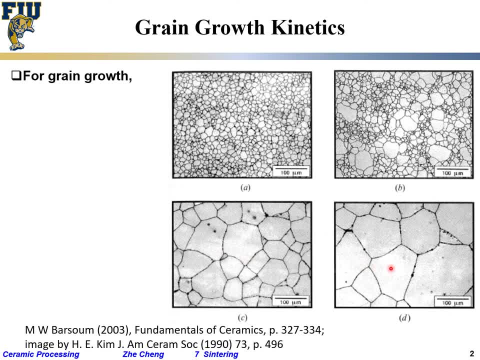 grows and grows and towards the end you will find that the green boundary become pretty flat and everything more or less on the same order of sizes. okay, and if green boundary is ideal and free of these defects, pores, inclusion and solutes, we would have the green growth roughly follows this type of relationship. 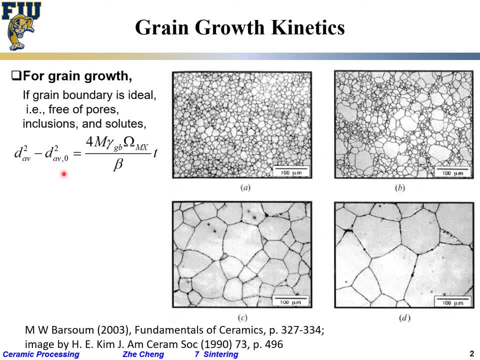 the average square minus the average time zero follows kind of still parabolic relationship: t, constant. here the whole thing is constant. okay, let's don't get into the detail: the surface energy, the volume for local, probably atom and other constants. the actual green growth or causing situation is complicated by 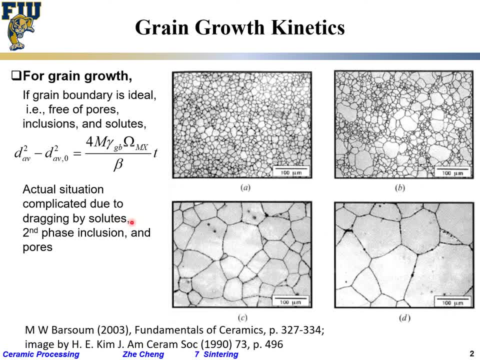 non-ideal system. you have solutes, foreign atoms dissolved in your material, you have second phase impurities, you also have porosities. so this model, people have to revise it. instead of having two here you can empirically fit people put an m here. the range of costs around two, from one something all the way to maybe three. 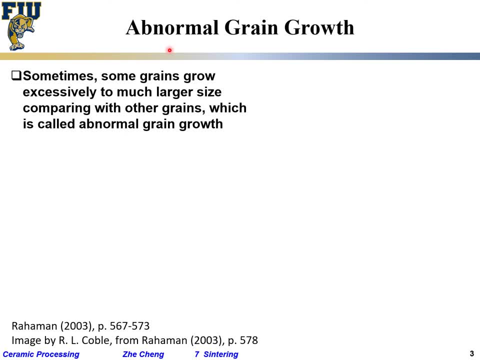 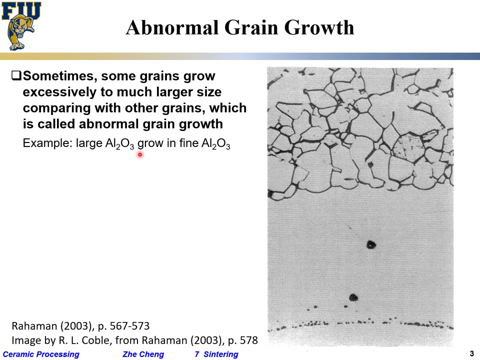 sometimes people observe so-called abnormal green growth. abnormal green growth which means certain greens grow excessively much, much quicker, much, much larger than all the other grains, and which is called abnormal green growth. and we have one example which is very large: aluminum oxide or aluminum grow in fine aluminum, something like this. you see, this side is the typical green, everything well. 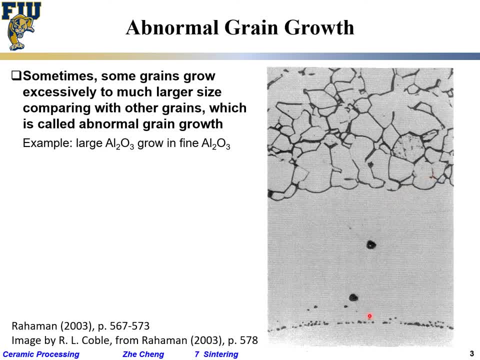 more or less comparable. but suddenly i have a huge, huge grain. this is called abnormal green growth. abnormal, suddenly, one green or few greens grow significantly, one order of two order magnitude larger than the other things. obviously you do not want this because in terms of mechanical uniformity here is very different. 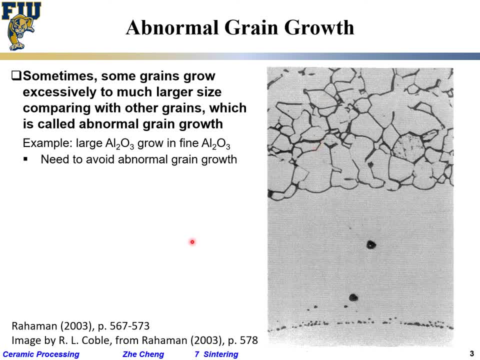 from here right, quite often, you want your material, you sell it, you want your material to behave more or less the same hardness. same toughness instead of one region much harder than the rest. okay, the origins, despite all these years, are still not completely clear, okay. okay, essentially i said nothing, but it's due to anomaly in green boundary mobility. 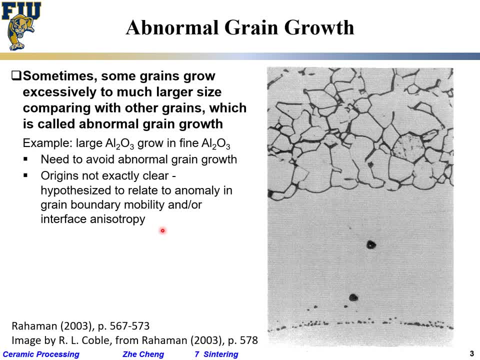 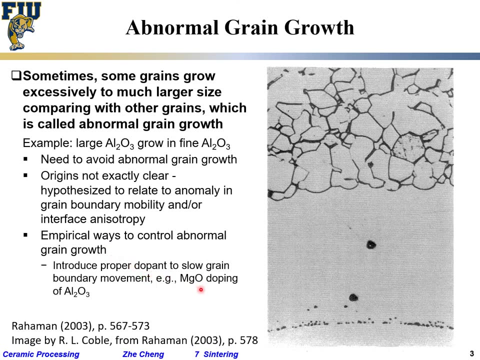 and the interface and isotropic. some of the interface is not the same versus the other interfaces. and to control or to try to avoid such things of normal green growth, you would try sometimes to introduce dopant to reduce the green boundary mobility, make it slightly slower, so that okay. 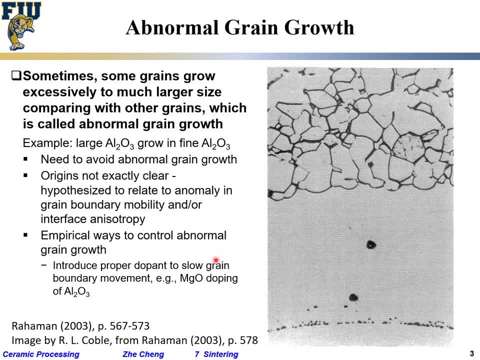 at least i can drag it down. not everything, not one local goes very fast. and you also try to eliminate so-called liquid phase because liquid, by its faster diffusion, faster mass transport will. if the liquid distribution is not uniform, you may imagine certain regions- it grows. 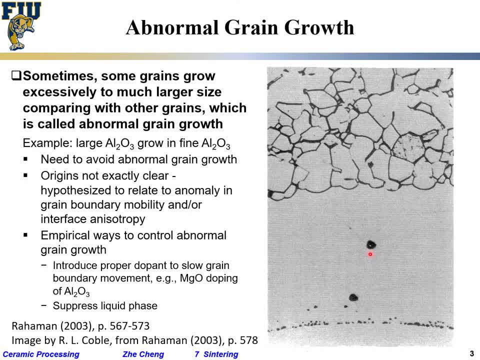 tremendously larger than the rest. if the liquid is not uniformly distributed, okay, and liquid actually will sometimes not distribute uniformly, because liquid also wants to shrink together to reduce the surface tension.